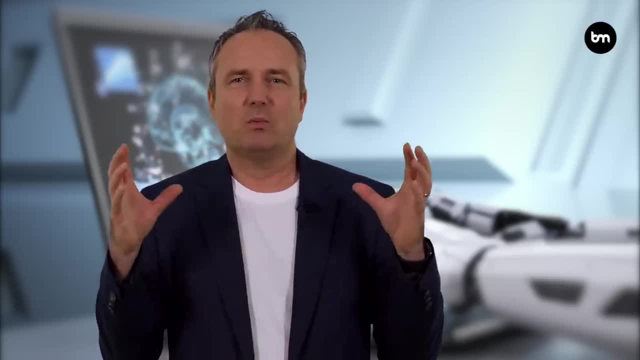 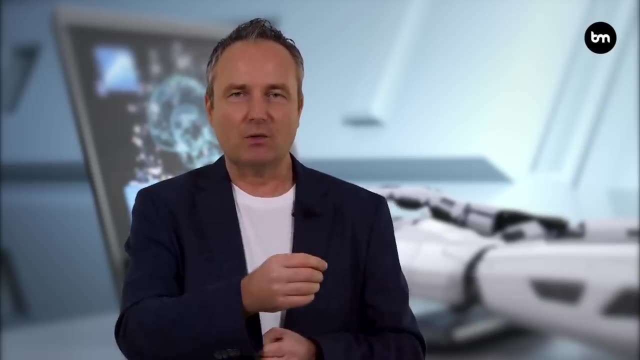 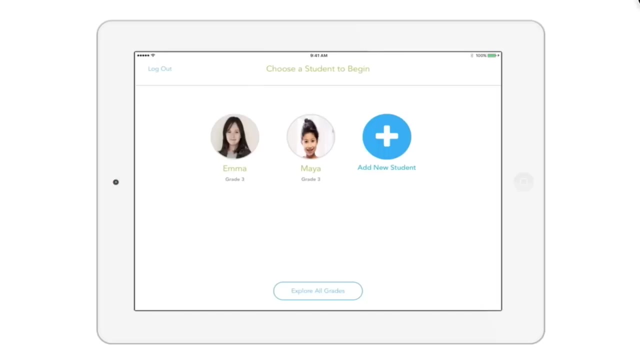 Content Technologies and Carnegie Learning that are developing these platforms, these learning platforms that enable AI driven learning, testing and feedback that students will get. Think about an app, for example, that enables you to learn math. So there's Thinker Math, for example, an app that will track student progress. They will 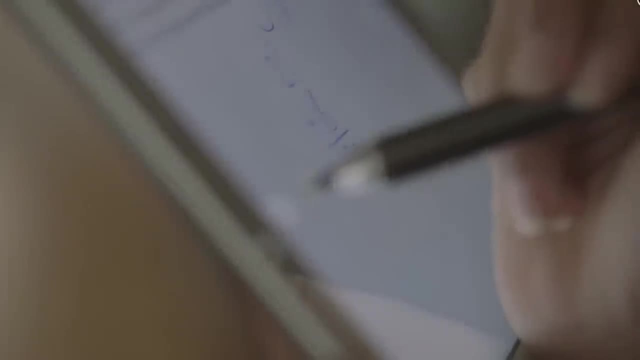 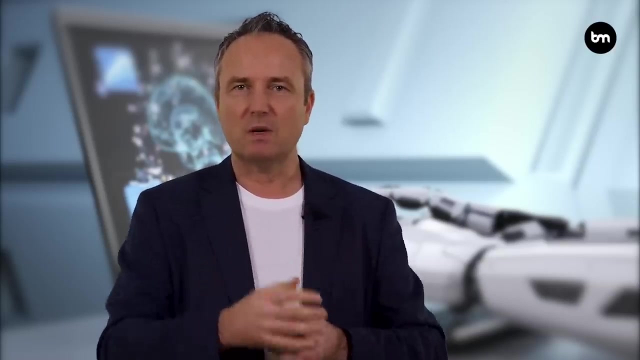 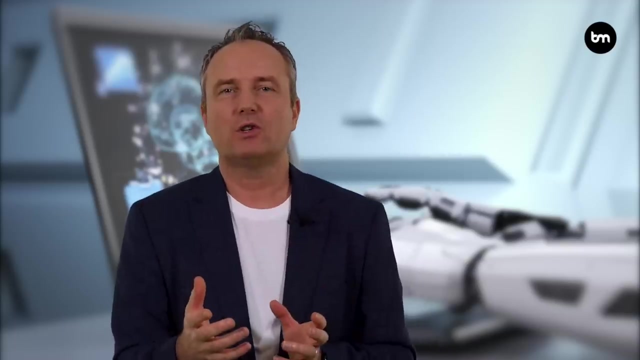 really identify areas that you are not particularly good at, and they will then emphasize and they will provide more learning on them. So the speed of every individual student can be customized, And this is something that a teacher simply can't do with a classroom of 20 or 30 children. We are already used to using these kind of approaches in language learning. 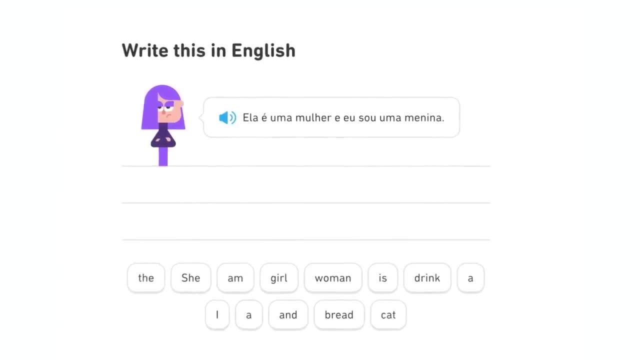 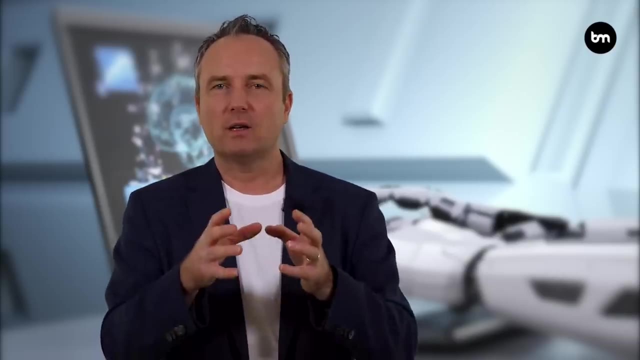 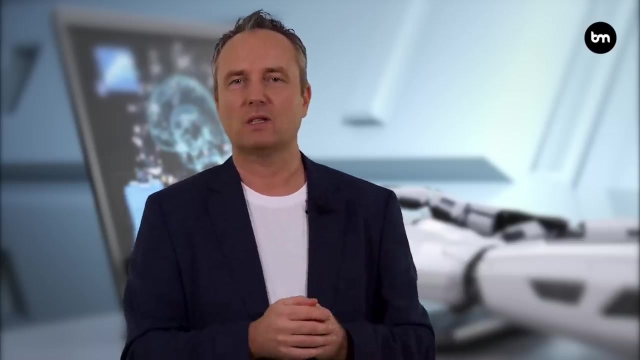 where we have tools like Geolingo and Bubble that basically allow hundreds of thousands of people to learn languages at their own pace. It will accelerate learning speeds or decelerate them and focus on certain areas that the AI will observe where they need more support And if you. 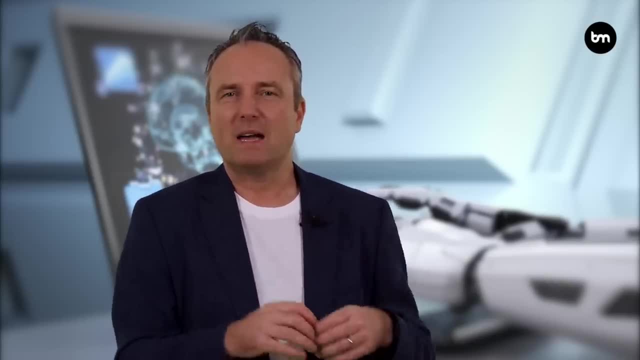 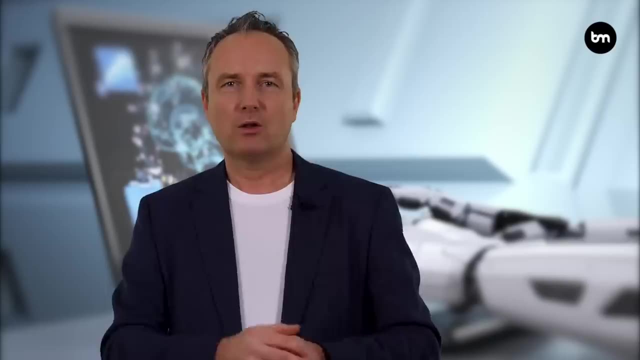 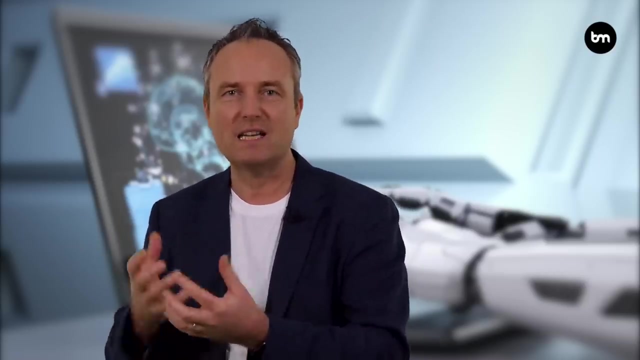 combine some of this learning where some of the very basic knowledge transfer that teachers have to do. you can outsource some of this to AI and then actually make the role of the teacher much more exciting, where they can spend time with students to do the really human, the interactive. 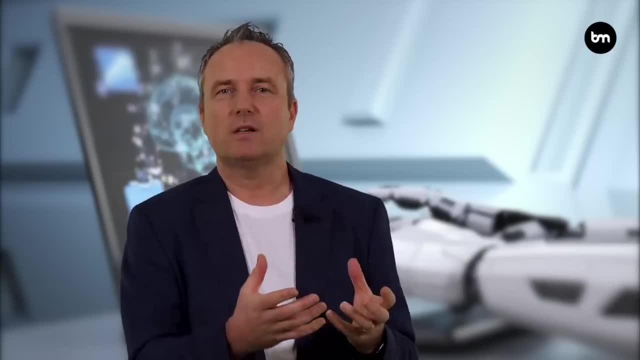 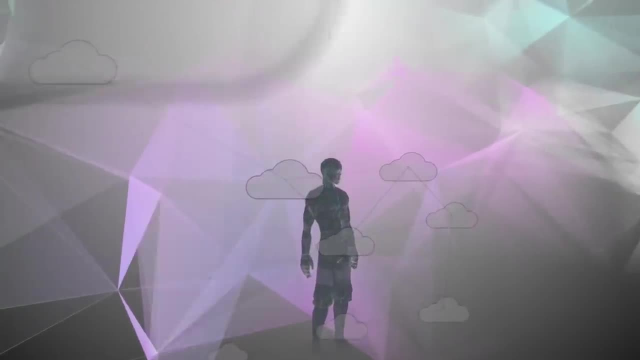 the creative part of the learning bit. So using artificial intelligence in education also enables us to potentially give universal access to learning. In the same way that we can use these apps in our schools, you can make them available worldwide, in any language and any student. 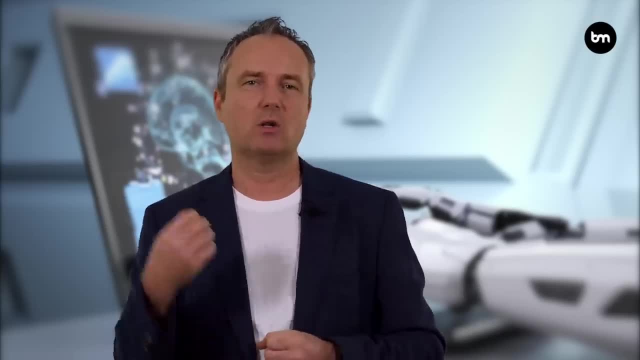 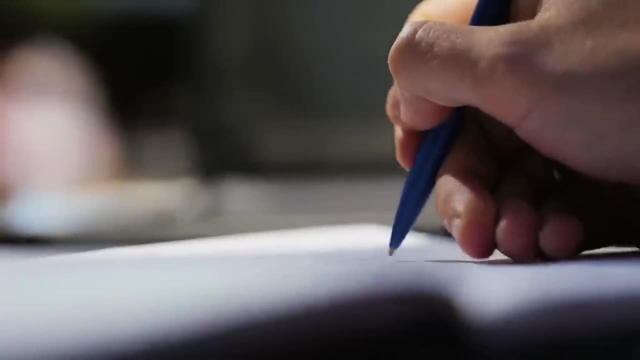 anywhere in the world can have access to the best language learning, the best math tutoring and so on, And artificial intelligence allows us to outsource some of the administrative tasks. We've seen this for a while that we've had the ability of machines to grade our multiple-choice. 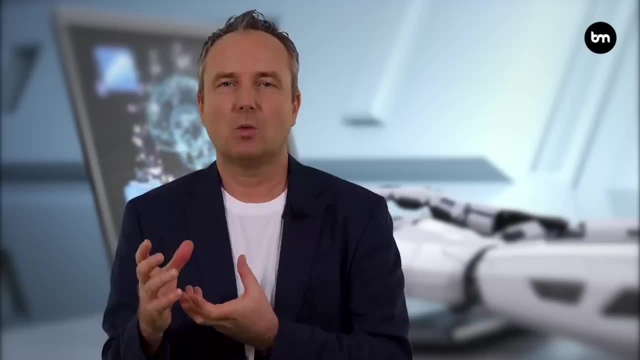 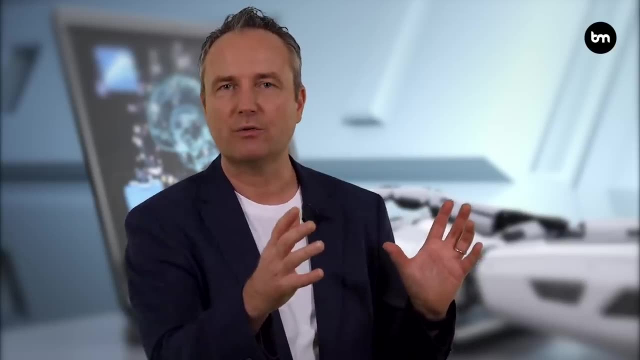 exams, for example. AI has come such a long way. Nowadays we have AIs that can write in their own language. We have AI that can write in their own language. We have AI that can jot down entire books autonomously, that can summarize entire libraries of books for us. So it 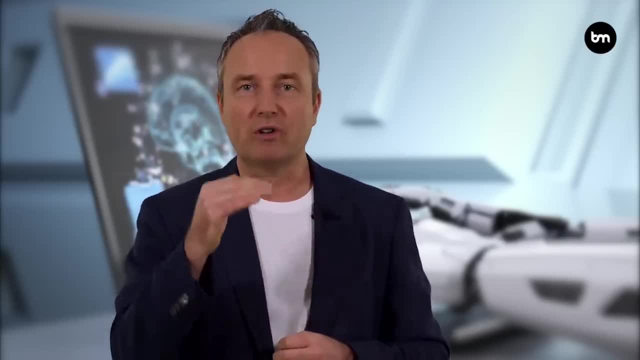 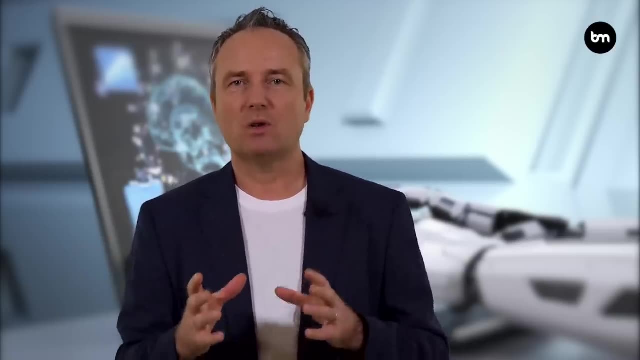 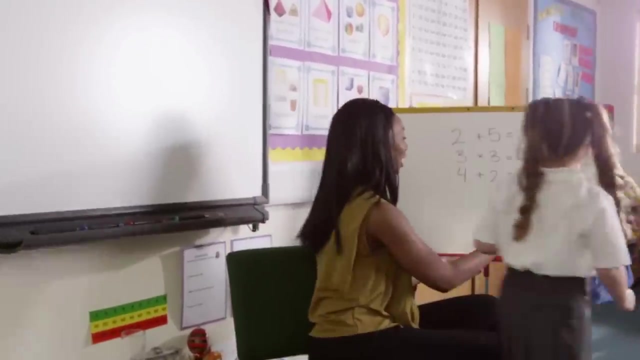 is not a big reach for them to also grade written essays for the people. So, again, what we're trying to do is we're trying to enable teachers who spend more time on the things that they love and outsource some of the more mundane administrative tasks to the artificial.